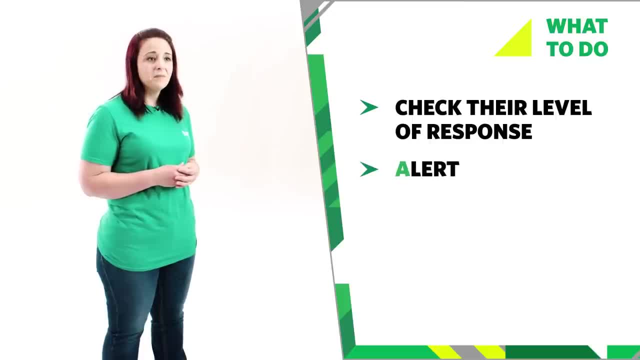 alert. Can they respond to you if you talk to them? If they only respond to voice, they will not respond to you. If they only are able to talk to you, they will. If you have any questions, leave them in the comments. 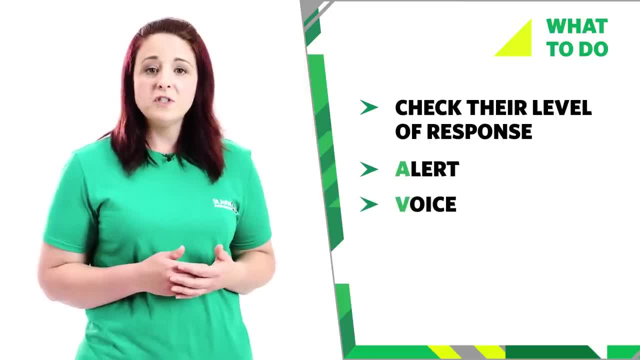 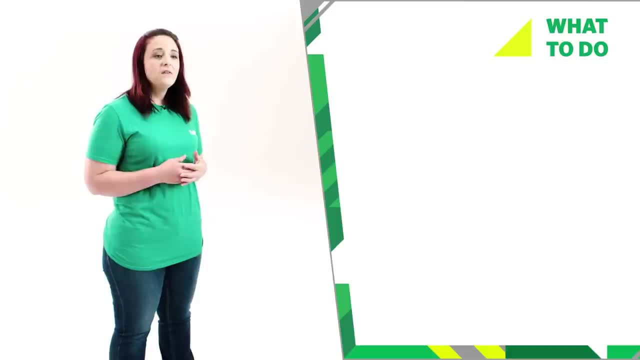 Thank you. they're drowsy. Do they only respond if you flick the bottom of their foot? Do they only respond to pain? Are they unresponsive to any of the above? If you are worried because they're not alert or because the injury is serious, then call. 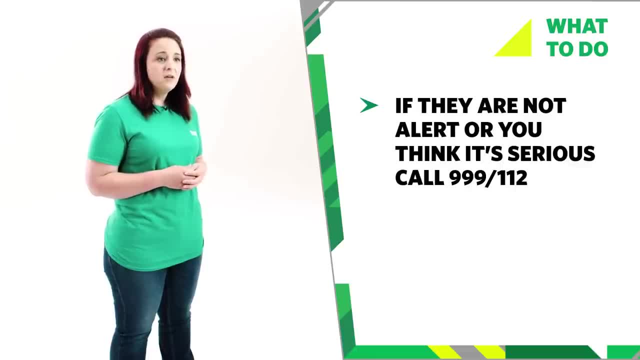 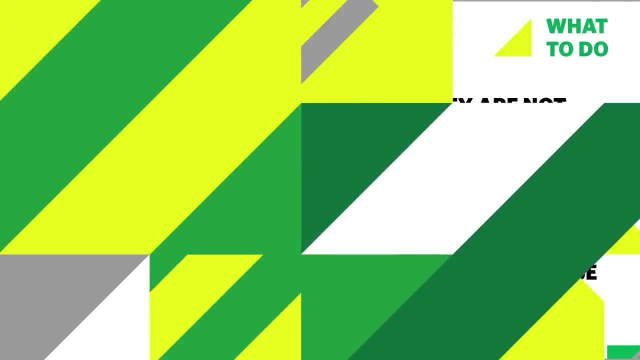 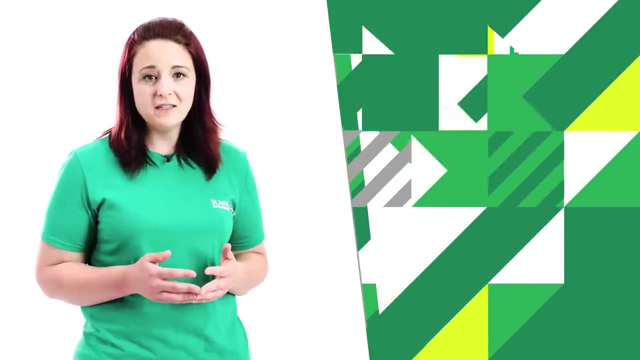 999 or 112 for emergency help. If they have any wounds, treat them by applying direct pressure to the wound and keep checking their level of response. If they've had a serious knock to the head, they may have a serious head injury and show some of these signs. They 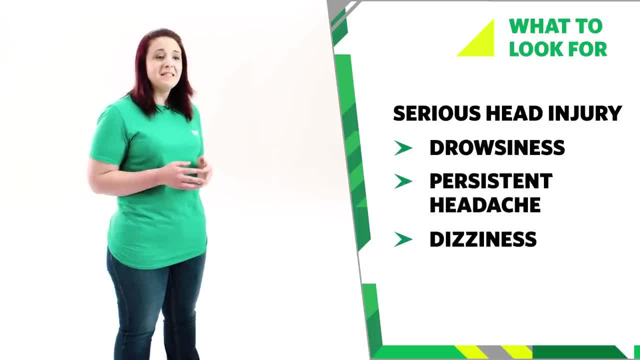 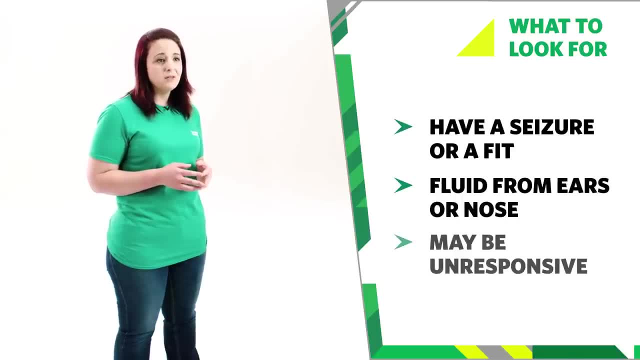 may be drowsy, they may have a headache, they may be dizzy, they may vomit, they may suffer a seizure or fit, there may be fluids coming from their ears or nose and they may be unresponsive. If you know that your baby's had a severe knock to, 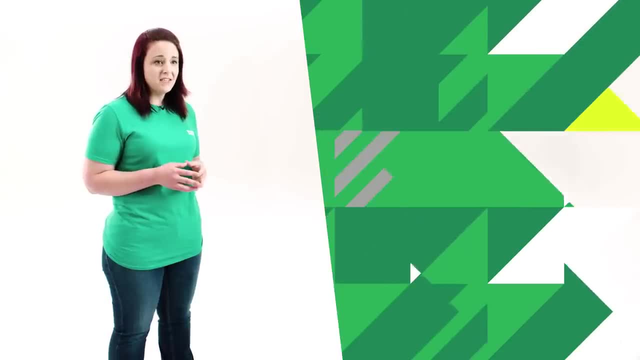 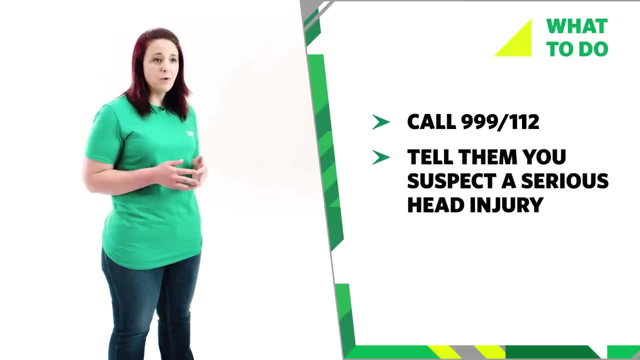 the head or you notice any of these signs or think they're getting worse, you should call 999 or 112 for emergency help and tell them that you've had a severe knock to the head. If you suspect a serious head injury to a baby while you're waiting for help to 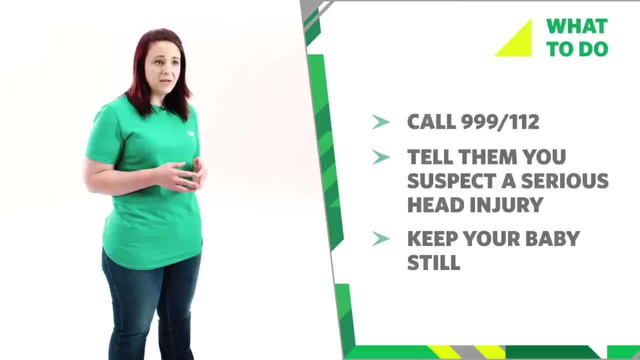 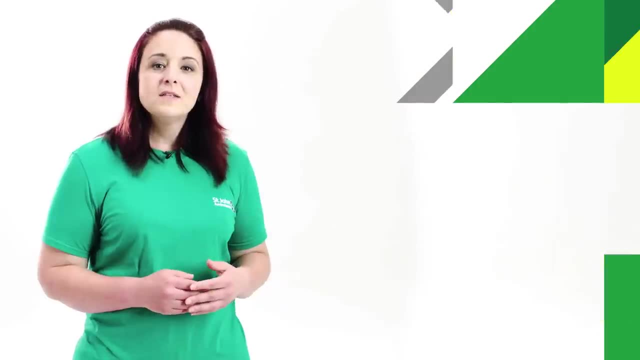 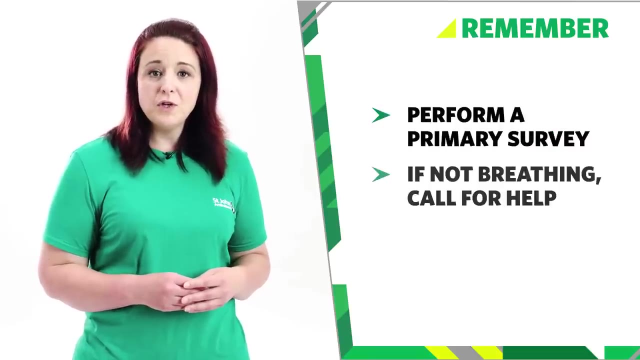 arrive. try to keep your baby still in case they've suffered a neck injury. Check your baby's breathing and prepare to start CPR if they stop breathing. So remember, if your baby's had a serious fall, perform a primary survey. If your baby is unresponsive and not breathing, call for help and ask a helper to call. 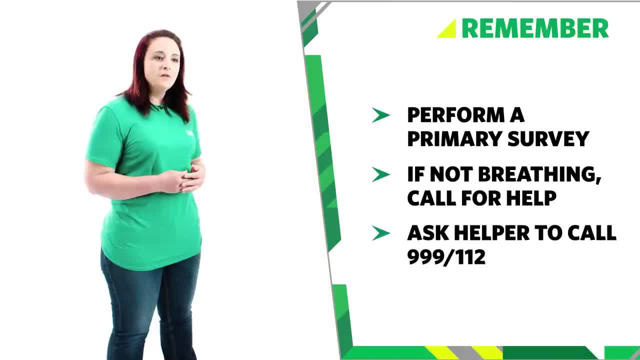 999 or 112 for emergency help. If you're on your own, use a mobile on speakerphone so that you can start CPR as soon as possible. If you do not have a speakerphone, do CPR for one minute before calling for emergency help. 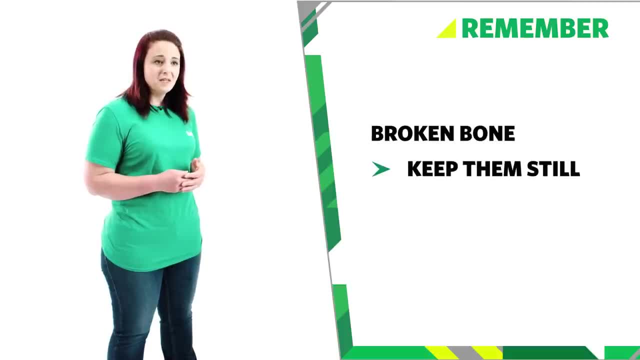 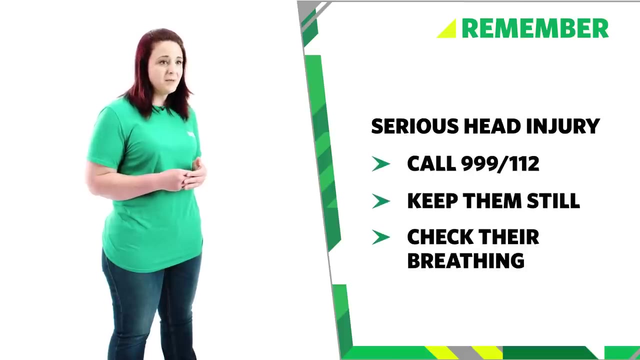 If you think your baby has broken a bone, keep them still support the limb and call 999 or 112 for an ambulance and keep checking their breathing and level of response. If you're worried or think that it's a serious head injury, call 999 or 112 and keep checking your baby's breathing and prepare to start CPR. if 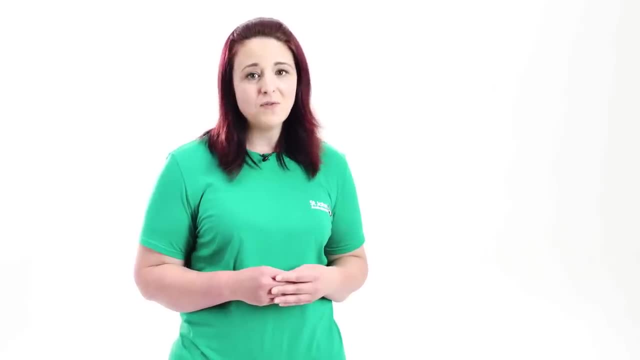 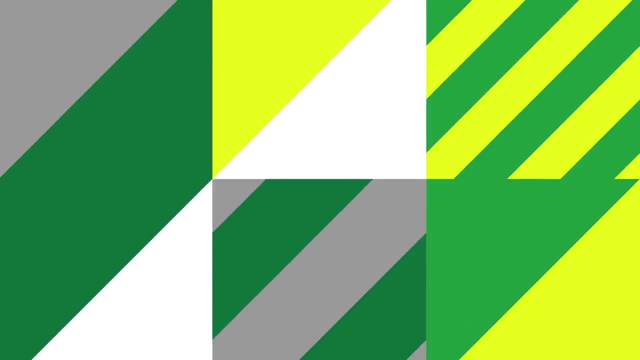 necessary And that's how you treat a baby who's had a serious fall. Thanks for watching. Help support St John Ambulance. Donate today.